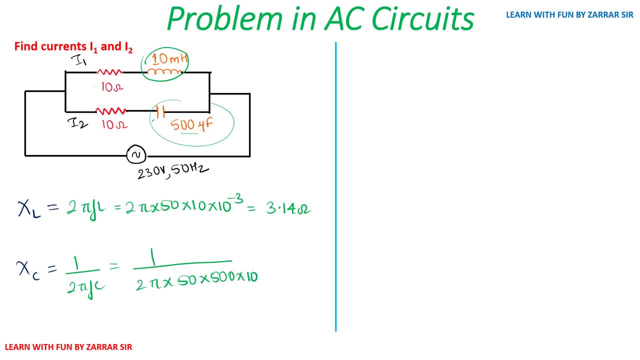 so i'll write 500 into 10, raised to minus 6, and this value will be turned out to be 6.366. okay, you can solve it later on. i won't waste your time, so i've already calculated for you. this is my xl. 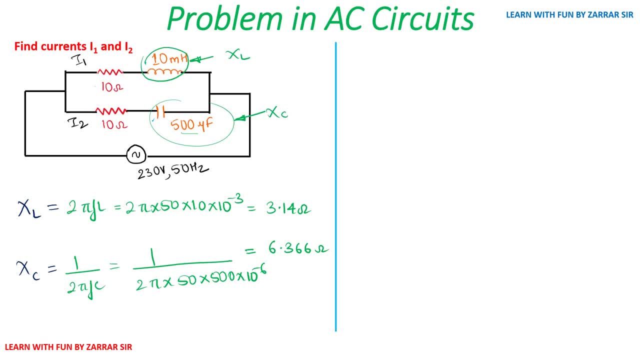 and this is my xc. okay, inductive reactance and capacitive reactance. now we will be understanding something very interesting, which will be my z1. i'm trying to calculate impedance of this small network. okay, so i'll be trying to calculate impedance of this small network. my z1 10, which is resistance plus c, will be converted into complex form: j. 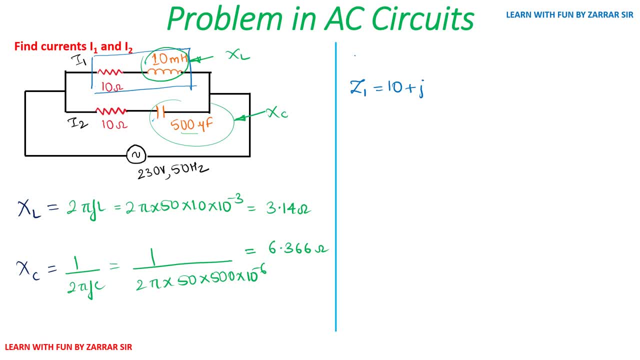 and you won't write this 10. please be cautious while writing. don't write this 10 milli henry. we have already calculated this 10 milli henry as xl and the value of xl is 2 pi fl, which is 3.14. 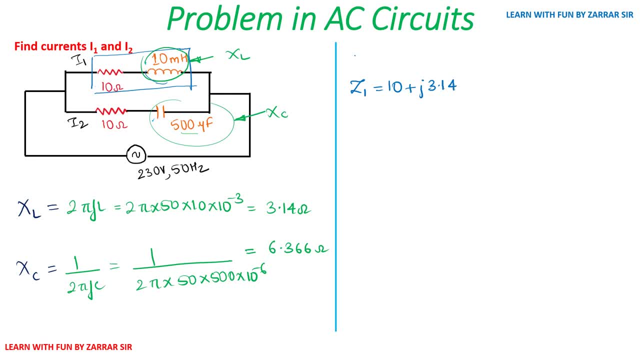 so i'll write 3.14. similarly, for my z2 i'll write 10, which is over here. so i'll be calculating this total resistance plus capacitance z i'm adding because they are in series. similarly these are also in series, so 10 plus. but remember for capacitor you have to write minus many student. 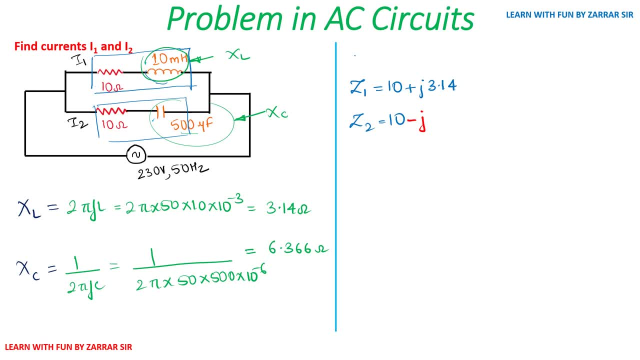 make a mistake over here minus j time, and the value we have already calculated for capacitance xc as 6.366, so i'll write 6.366. now the value which i have written of z1 and z2 is in rectangular form. i'll be converting into polar form. so to convert into polar form i will. 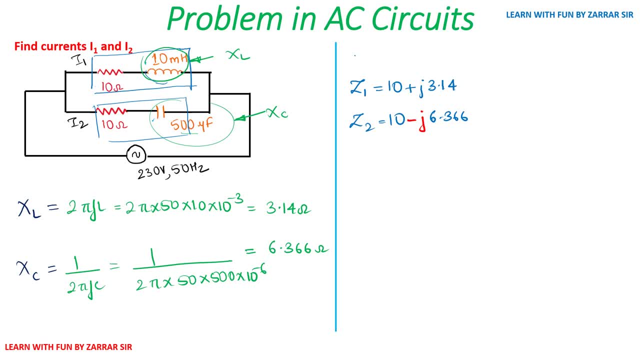 not be calculating or wasting your time in calculation, but i'll guide you how to do it, because many student ask how to do it. see, to calculate, this is rectangular form. to convert into polar form, you will just use this value as a square plus b square, so this will be 10 square. 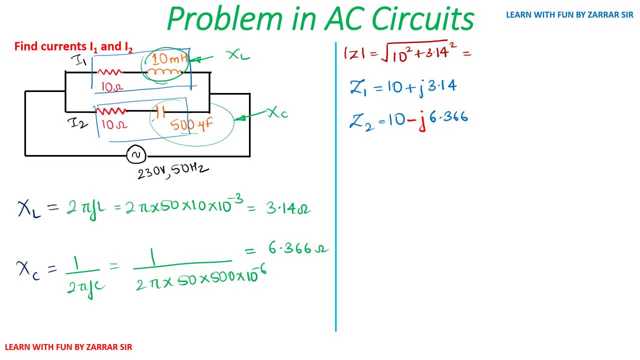 plus 3.14 square, and you will get the value of z, which will be turning out to be 10.48. okay, similarly, to calculate angle, the formula is theta: tan inverse of b by a. okay, b by a means. 3.14 divided by 10, you will get the value of tan inverse, which turns out to be 17 degree. 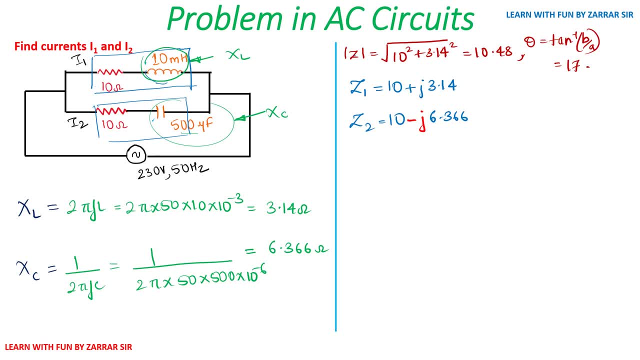 okay for this problem, for z1. so you will be 17.43 degree you will get. once you get this, you will substitute over here. okay, so i have converted rectangular into polar form and how you will write polar form. you will write it in this way: 10 point. okay, i'll use some different colors because 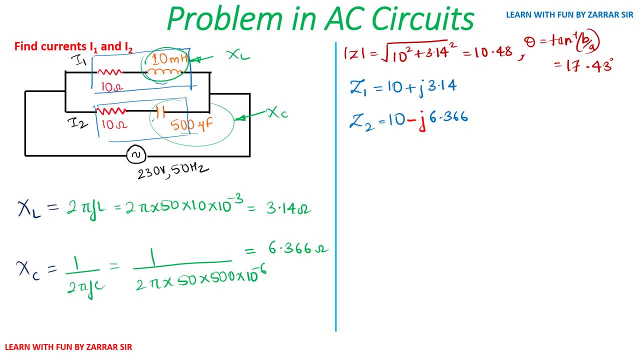 this is very light, okay, so let's have some different color. let's take red. okay, it is 10.4, 48 angle, 17.43 degree. similarly, if you use this above method to calculate z2, you will get the value in polar form as eleven point four, eight, sorry, eight, five, eleven point. okay, should use. 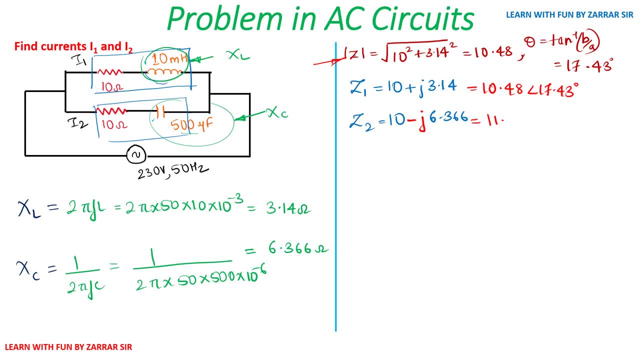 eraser. it is eleven point eight five and the angle is over here. that's minus thirty two point four, eight degree. this both are impedance, so the unit will be ohm. so now you can understand. i have converted the capacitance and inductance in the form of reactance and i have combined it to calculate impedance. so under basic the thing, 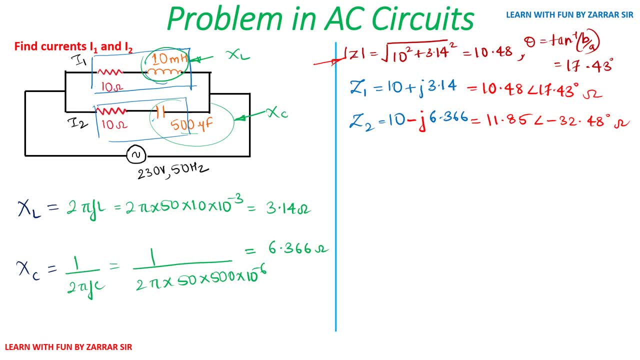 what i have done is i have converted- remember the step- i have converted inductance into reactance and finally, i have added this reactance with resistance and i'll name it as impedance- okay, z1. similarly, capacitive reactance: xc plus resistance. this will give me another impedance, which is z2. 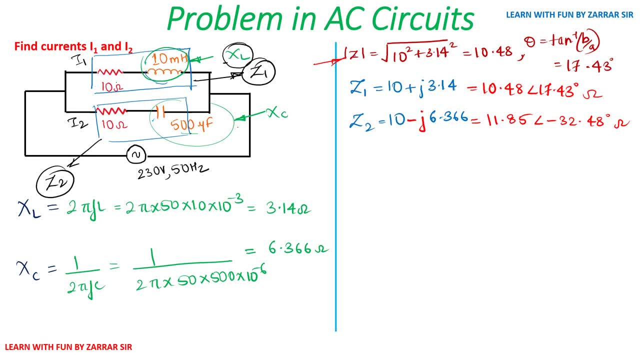 so i've calculated z1 and z2 and my task is to calculate i1 and i2 and we know the fundamental ohm's law, v equal to ir. so my i1 will be v upon r1, right guys, v upon r1. what is my v? my v is this: total voltage, 230 volt right and 50 hertz, but i 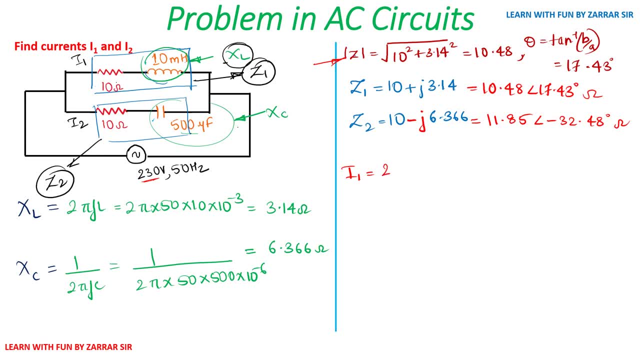 don't have an angle. so no, don't worry about this, just write the basic v upon z1. okay, so i'll write v upon z1. what is my v? total voltage: 230 volt. okay, but i'll should write it into angular form. since i don't have any angle, i'll write 0 degree, so 230, angle 0. 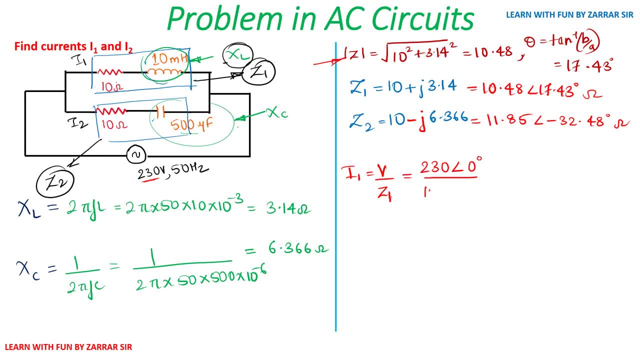 divided by 10.48, up angle 17.43. now how to solve this? this is very simple. just divide the value with the value and angle. while solving angle, make sure you subtract, please it okay, so i'll guide you how to do. is 230 upon 10.48. once you solve this, you will get 221. 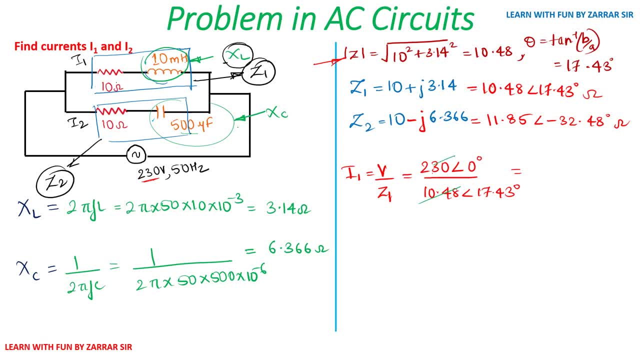 so you have to solve this. by this you will get 21.48. sorry, 21.95, i've just calculated it- an angle- make sure, angle, you don't divide it. you have to subtract, okay. so numerator minus denominator. so 0 minus 17.5, 17.43 will turn out to be minus 17.43 degree. so this is your current. 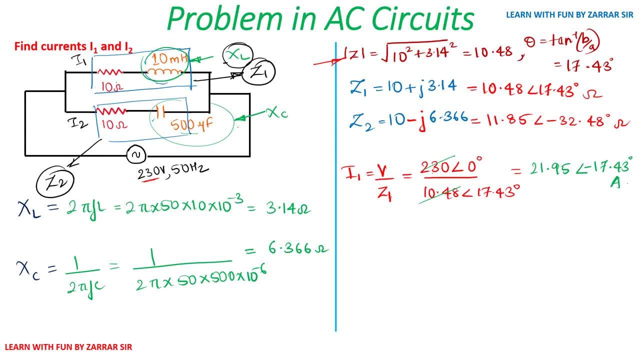 and you know the unit of current is ampere. similarly, we'll calculate i2. so how to calculate i2? v upon z2? v is 230, angle 0, divided by z2, which is 11.85 angle minus 32.48. now you can say how to solve this. just divide 230 with 11.85. the value is